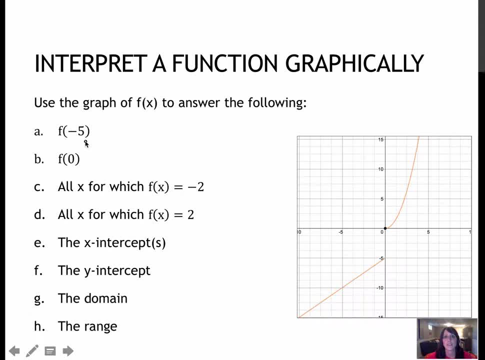 questions. So finding f of negative 5 is saying, if I plugged in negative 5, what would come out? If I look at that graphically, I'm just going to go to negative 5 on the x and find what's the value of y. In this case it would be. 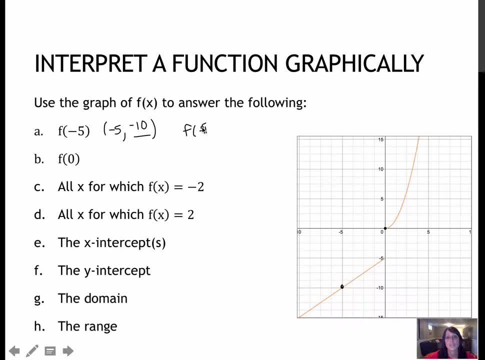 negative 10.. So f of negative 5 would be negative 10, because negative 5, negative 10 is a point on this graph. F of 0 would be when we're at 0, what is the value of the function? So 0 is one of those. 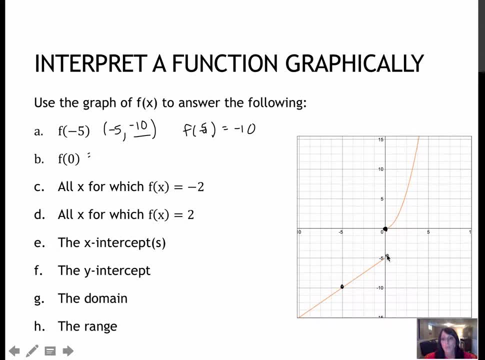 tricky ones, but here I've got the point at 0, so it wouldn't be here. This would be like that open circle, meaning f of 0 would be 0. This one's saying all x for which f of x is negative 2.. So in essence it's saying what x value would give you. 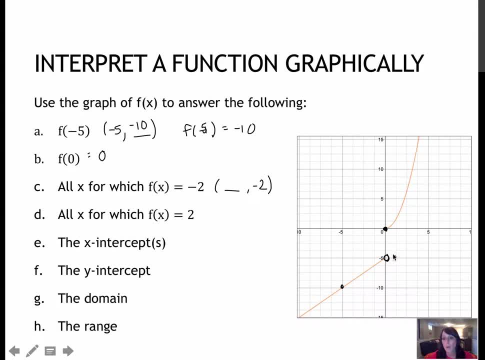 negative 2 as a y value. So, looking at my y, I'm looking at negative 2, and I see that there's no value at negative 2.. So this would be none or undefined, but positive 2 is here and that would be about right here. So I don't know an. 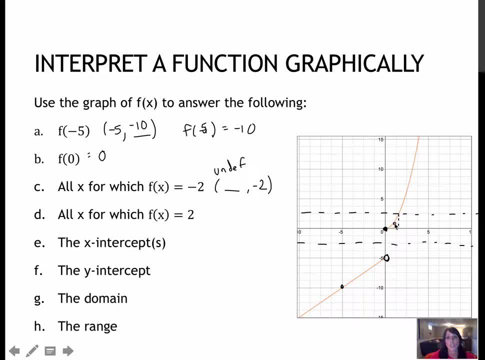 exact answer for that, because I don't have the graph, So here I'm just going to say about 1.1.. So obviously we don't like to round in mathematics when we don't have to, but I'm not really given an exact value and that was my fault, for. 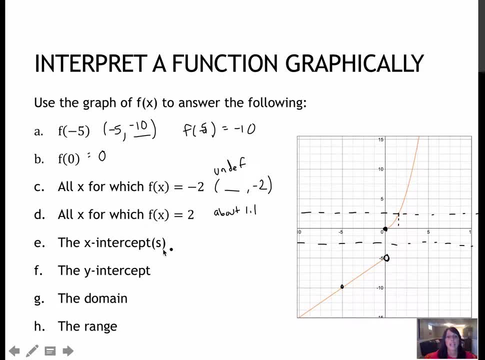 making that particular value on this question. The x-intercepts would be, of course, where does the graph, if anywhere, cross the x-axis? and here, that's at 0, 0.. The y-intercept, again, where does it cross the y-axis? also just at 0, 0.. So on. 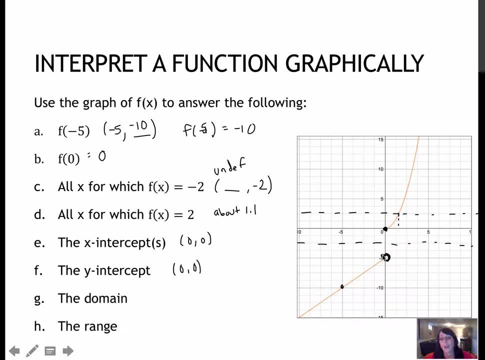 this one. it's not actually crossing, it's coming up to it and not quite touching it. The domain would be all of the x-intercepts and that would be the x-values that I can use. This would be everything. We talked about this in our 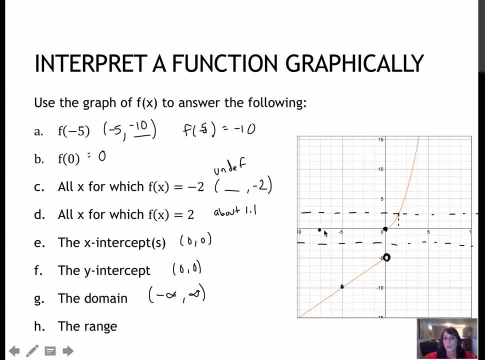 last questions. So everywhere on x I've got a value for y. The range, however, would go from negative infinity on the y up to 5,- sorry, negative 5, and then add to that starting at 0,, which again is a closed bracket, up to positive infinity. 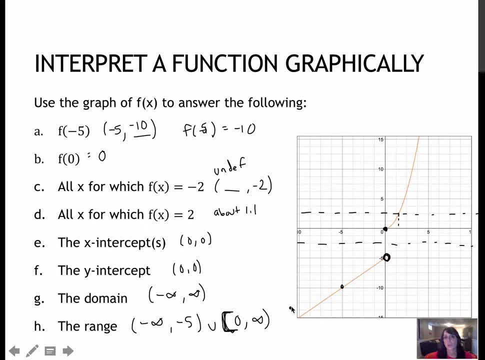 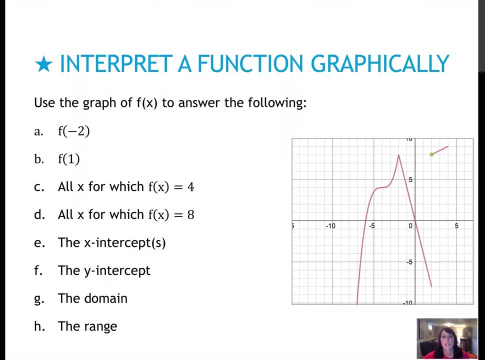 So it's kind of putting together a lot of stuff that you sort of already knew. This will come into play if you take, you know, a trig or a calc course. This is one for you to try on your own. So press pause, do all. 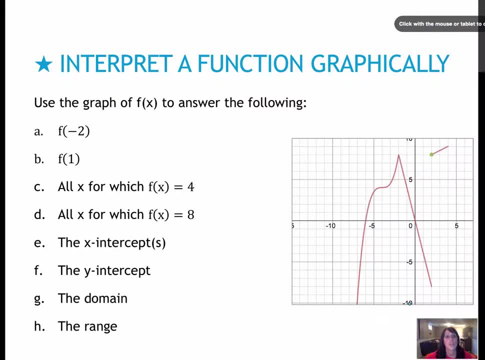 of the questions, then press play to check your work. So f of negative 2 means I'm going to negative 2 and finding what is the value. So that value looks to be positive 8. And for f of 1, it looks like 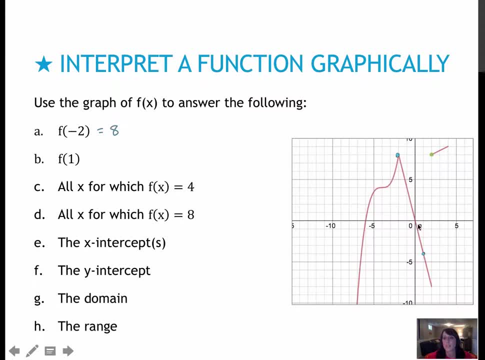 I'm down at negative 4, which means it's the point. The next two questions are basically saying: if y is 4, what's x? Or if y is 8, what's x? So if y is 4, I've. 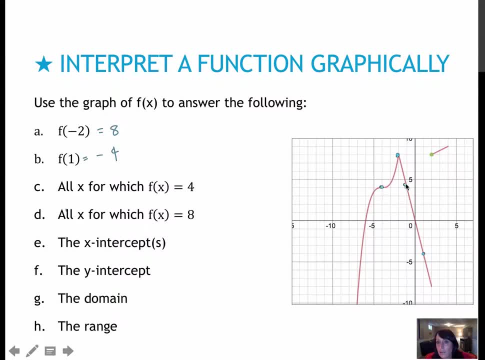 got a value both here and here. So if y is 4, then x was negative 1 or negative 4.. And if y is 8,, x was negative 2.. So notice, here I've got my negative 2 for 8 and my negative 2 for. 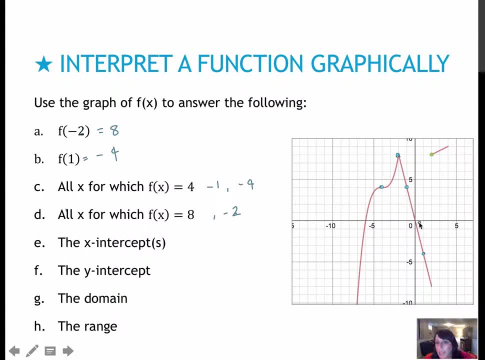 8, so it's the same point. The x-intercepts would be at 0, 0 and at negative 6, 0.. The y-intercept is just at 0. The domain, it looks like, goes from negative infinity, because 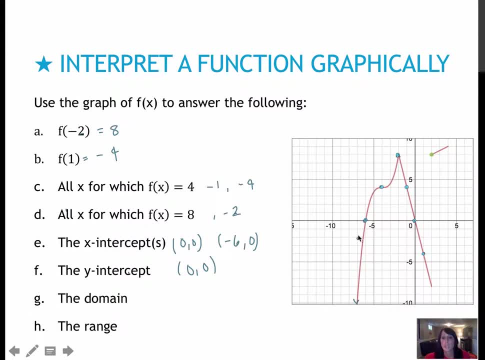 even though we can't see it. this line goes on forever and ever and ever. So any value I plug into the left is going to give me a value for y, But it looks like it stops right here at 4.. It's unclear if it's open at the end or not, so we'll assume that it is So. 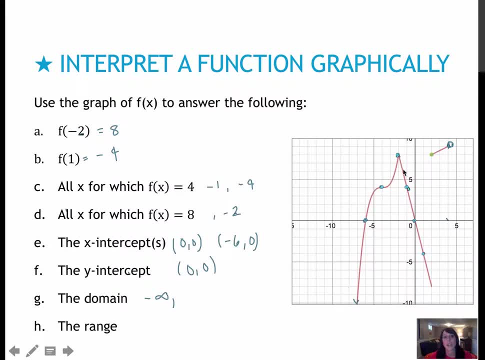 the domain would be from negative infinity. And notice, I've got a value all the way through up until I get to 4.. The range is The y-values, So the y-values the lowest is negative infinity, because it would just keep going down. The 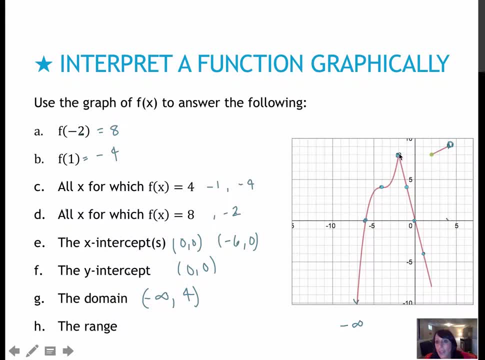 highest. I've got a high value here of 8, but over here I've got a high value of 9.. So it looks like from negative infinity up to 9, but not including 9, because we're going to assume that's an open circle. 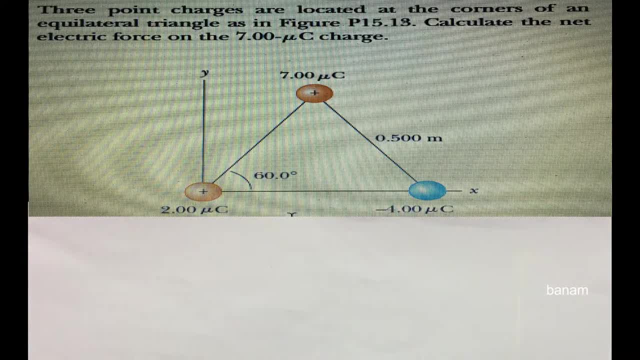 3-point. charges are located at the corners of an equilateral triangle, as in figure. Calculate the net electric force on the 7-micro Coulomb charge. Let us draw the equilateral triangle. Let us take the charges are placed at the corners. 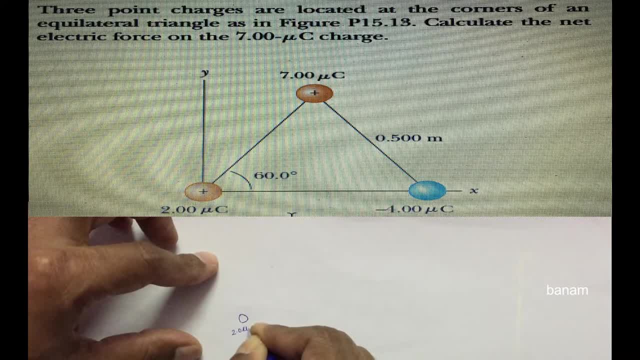 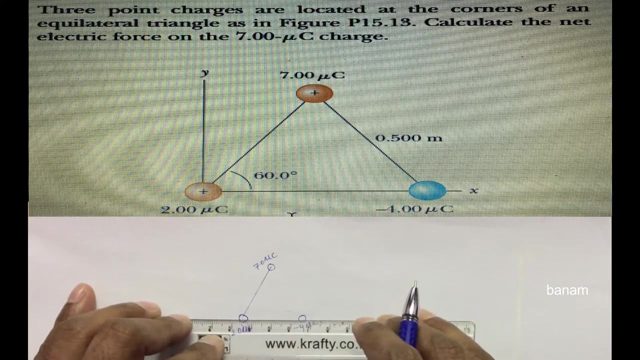 of the equilateral triangle. 2-micro Coulomb charge and minus 4-micro Coulomb charge and 7-micro Coulomb charge are placed at the corners of an equilateral triangle. The distance between the any two charges is the same and the angle between the any two charges is the. 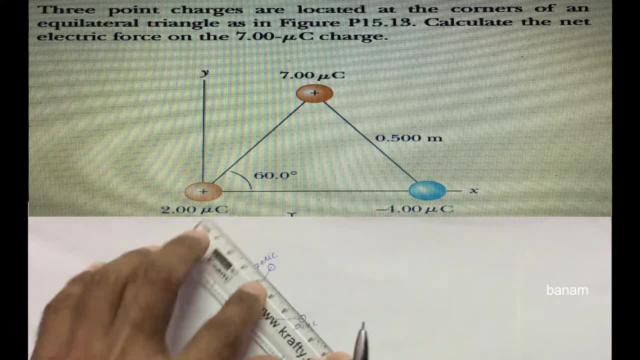 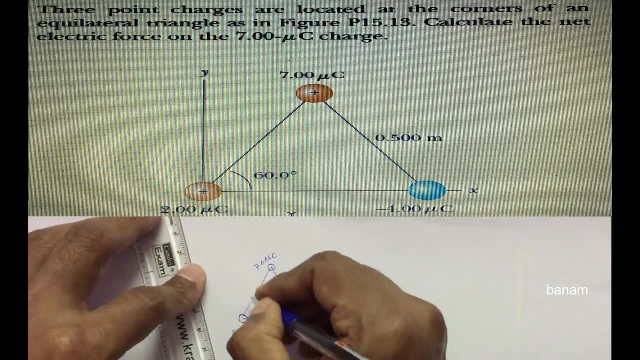 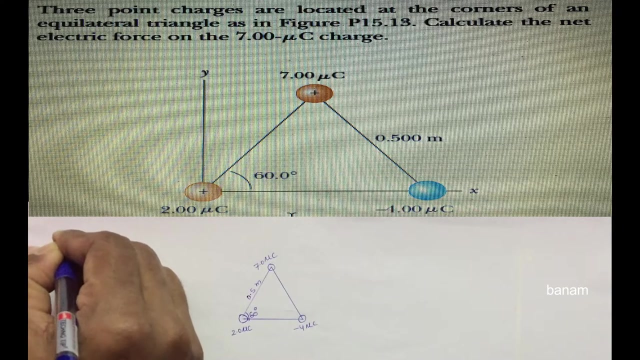 same Because the triangle is equilateral, the distance between the two charges is equal to 0.5 meters and the angle between the any two charges is 60 degrees. Let us take: Q1 is equal to 2.0-micro Coulomb charge. 1-micro Coulomb is equal to 2.0-micro.